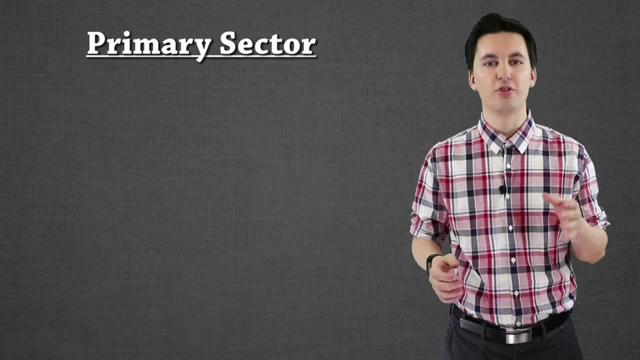 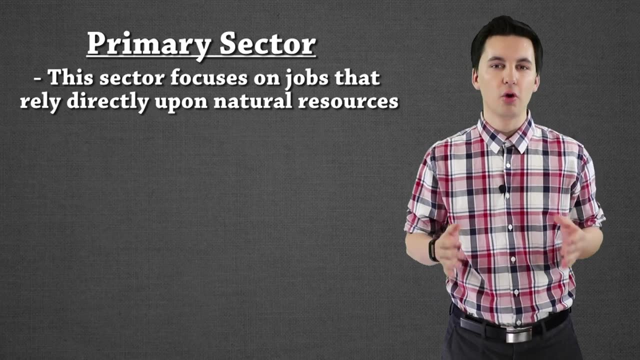 you understand the main concepts. Our first economic sector is the primary sector. Now think of this as kind of stage one. This is us gathering resources. So people who are in this part of the economy are going to be people who interact directly with each other. So if you're in the 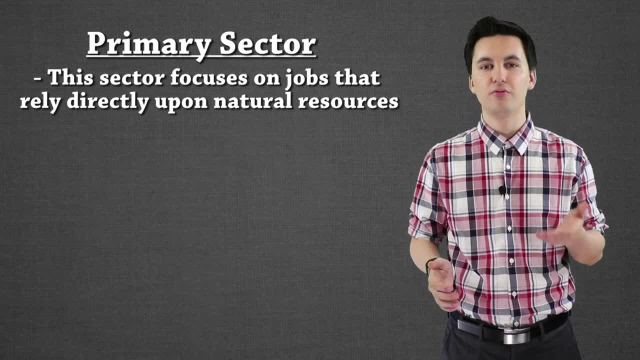 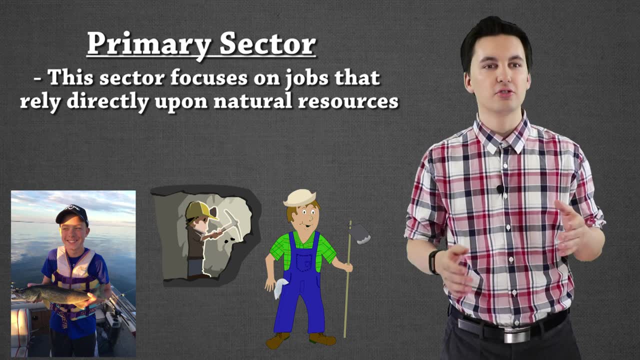 environment. this would be fishermen. This is going to be coal miners, people who are farmers. They are harvesting, They're collecting a resource, and so they are going to be dependent on that resource. They're going to be located close to whatever resource they'll be using, because 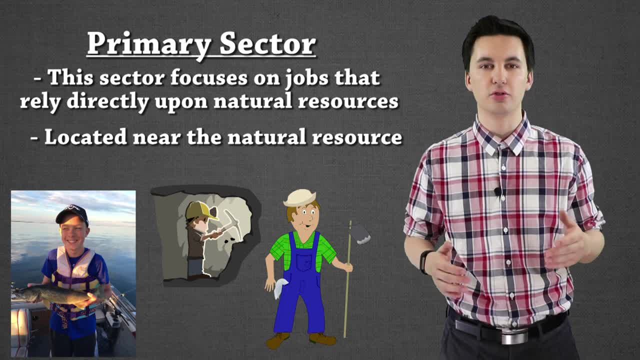 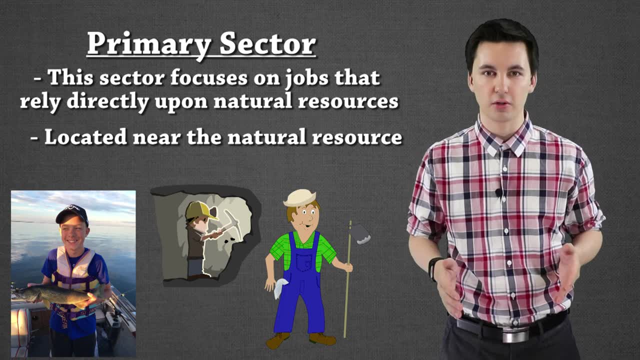